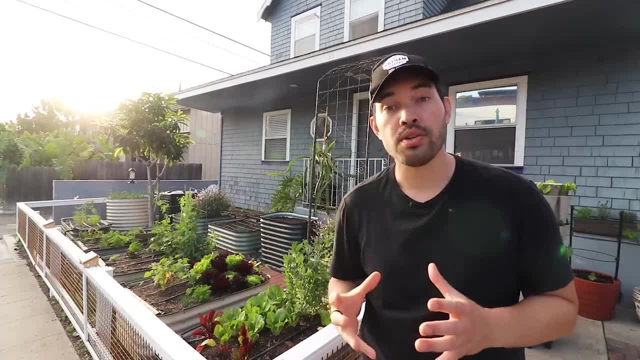 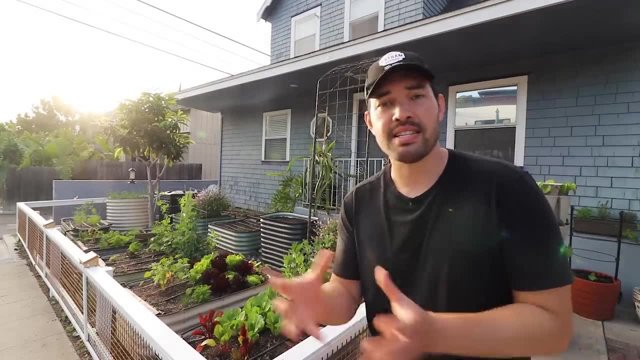 South is going to be the direction you want to expose your garden to, because most of our annuals and perennial vegetables that we grow prefer full sun, which means at least six to eight hours of sun, direct sun- a day, And so, as you can see, that's West. 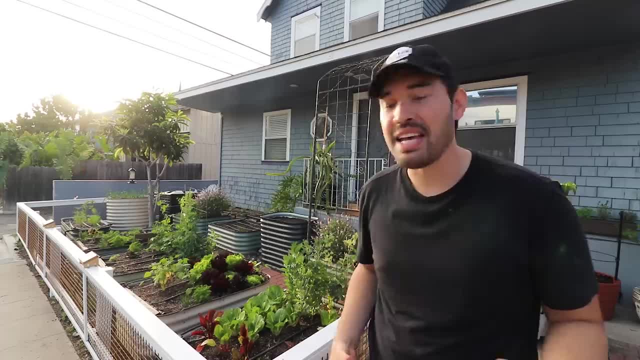 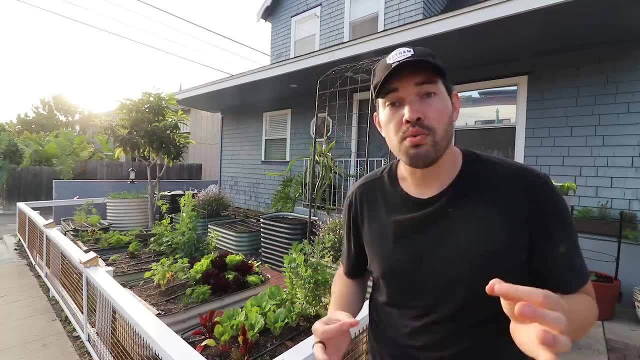 The sun is setting in the West right now in this beautiful, beautiful summery day here in San Diego, And I'm getting exposure throughout the whole day. So just like this, and it's a perfect, perfect amount. Now, if you mess this up, 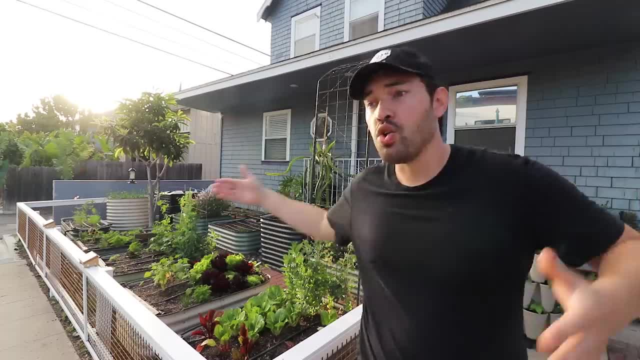 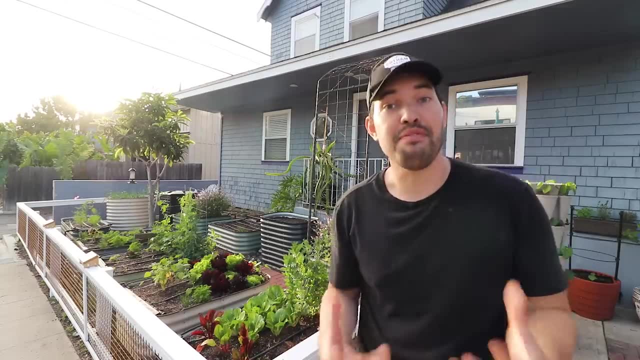 if you build your garden in the wrong place, let's say on the North side of your house on a tall wall, then you've just basically created a shade garden and you have to plant accordingly. Now I have a video on how to plant a shade garden successfully. 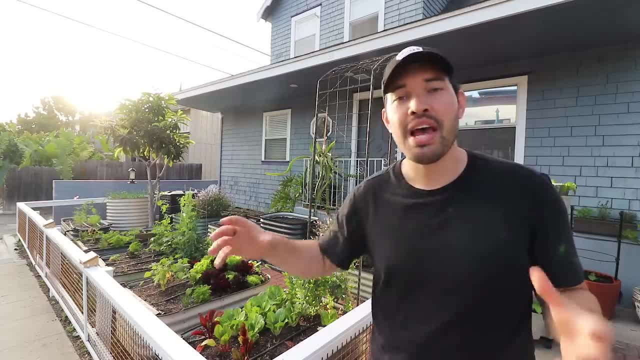 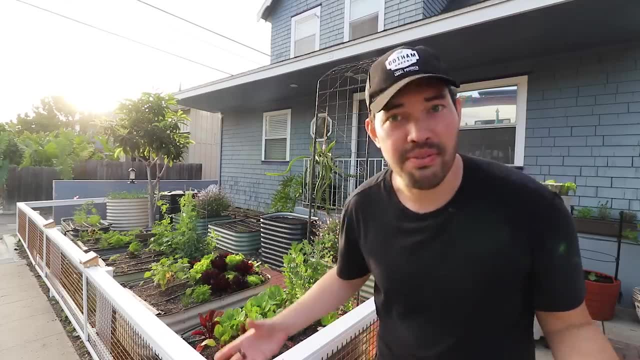 but you might not want to do that. You might want some Epic tomatoes, some peppers, all those classic things that want that sun. So what I would say is, before you place your garden for the year or for the rest of your life, honestly go and monitor your space, Come out and say okay. 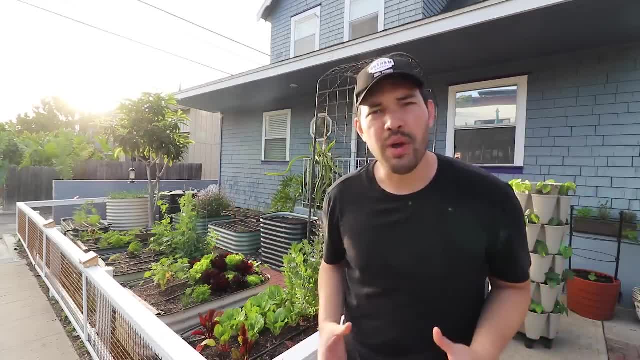 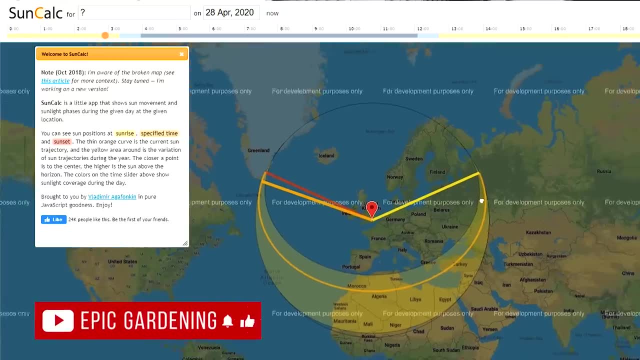 how's the sun falling? Is there a tree blocking me? What's getting in the way of my garden And, if so, plan for that? There's a really helpful website called suncalcnet, I believe, where you can actually scroll. 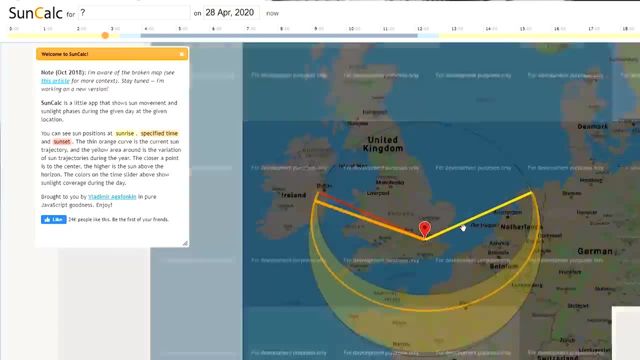 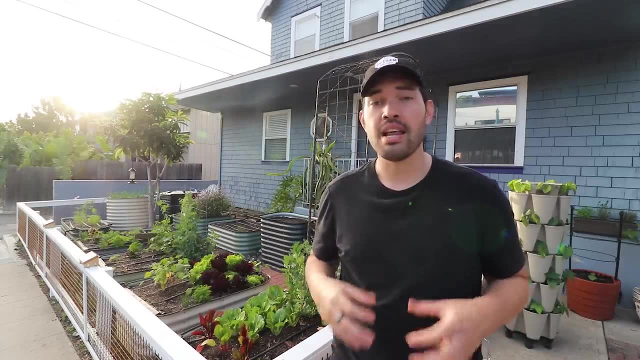 look around and on your exact GPS located property, you can see how the sun falls throughout the whole course of the year. It's a very helpful tool. So really do not make this mistake, because it is the principal mistake. Every other mistake is less severe than this. 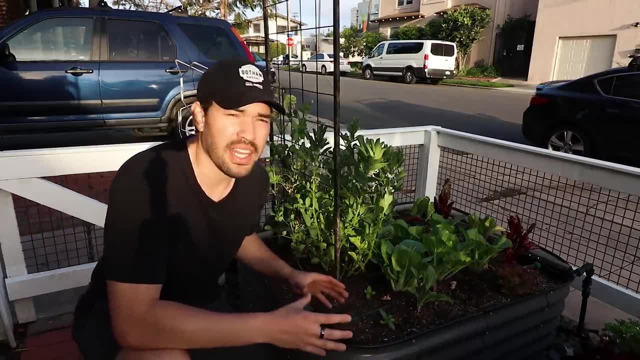 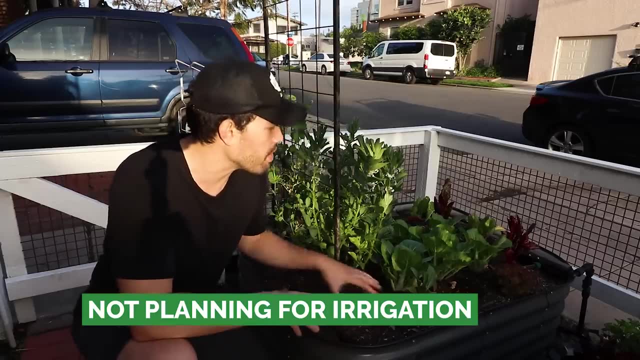 Another mistake that is very often made is not planning for irrigation. Now. there's many different ways to irrigate a garden and we can go into that in a future video. As you can see, I've done drip irrigation on mine. I have a whole video on how I set mine up, because it's a little bit extra. 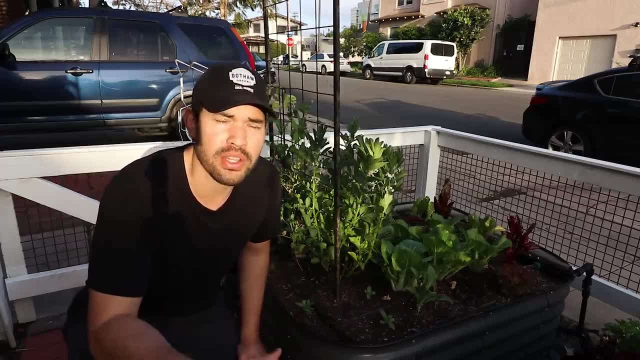 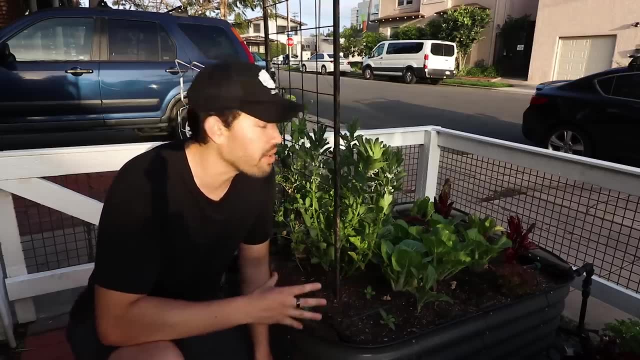 That's a little intense, but you need to plan for how you're going to irrigate, And if your plan is just saying, Hey, I'm going to come out enjoy the garden in the mornings with my cup of coffee, do a little bit of hand watering. There is absolutely nothing wrong with that. 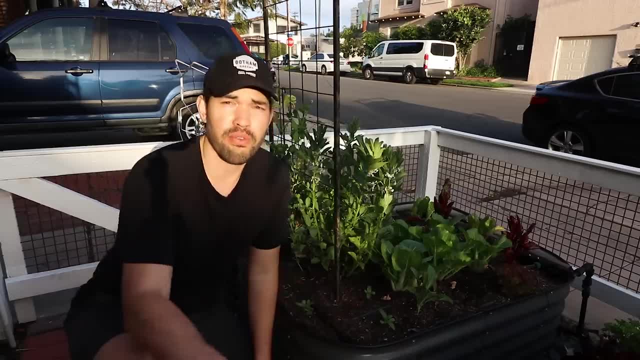 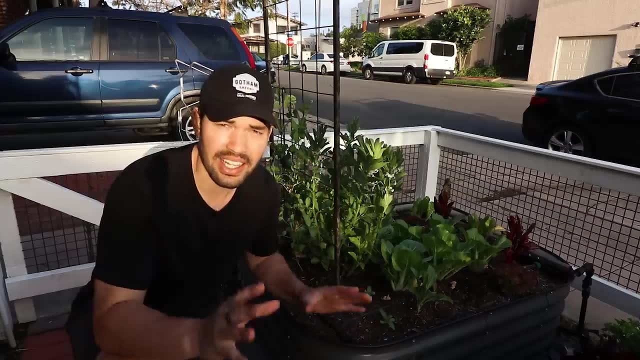 So long as you know, that's your plan, Because I'll tell you one thing: I've had to retrofit this entire garden with drip irrigation twice and it was not a fun chore. So with just a little forethought and a little planning, it would have gone a long way. Mistake number four: 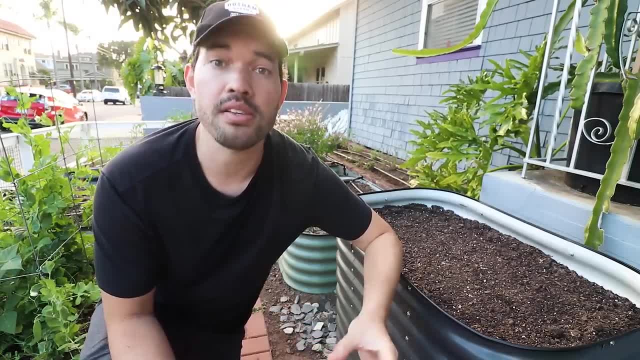 I almost do not want to confess to you guys, but I'm still going to do it because I'm an honest, upstanding gardener and I'm willing to admit my mistakes. So when I first started the Epic Garden, I ordered three and a half cubic feet. 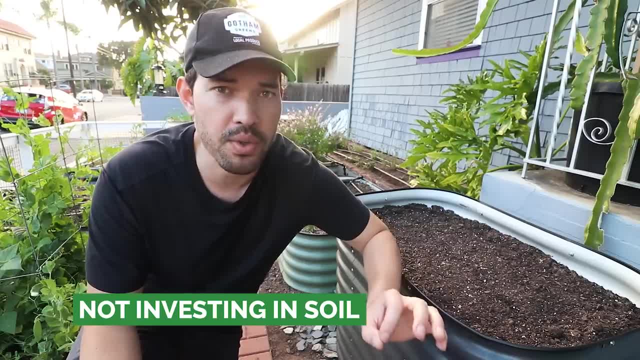 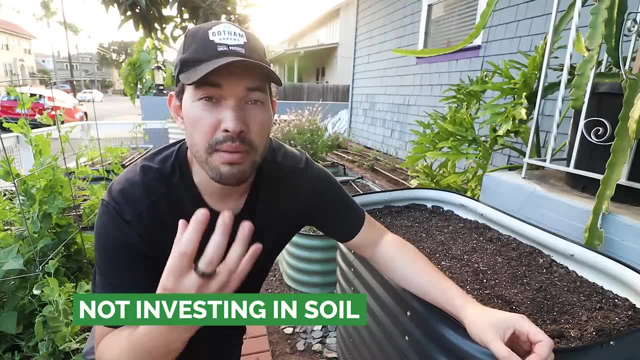 cubic yards- excuse me, cubic yards, which is a driveway full of soil. I ordered it and it was complete garbage. It really was trash. and it was supposed to be a high quality raised bed mix and it was not. It was basically full heavy clay topsoil with like a smattering of compost in it. 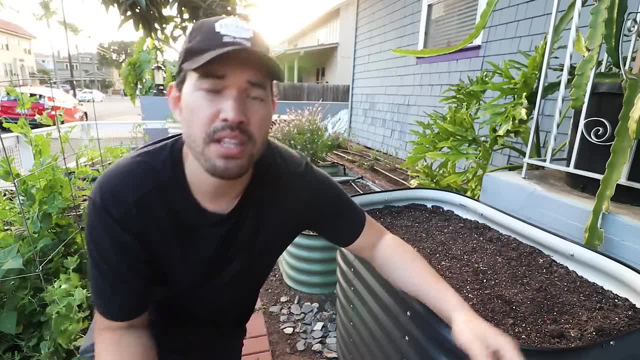 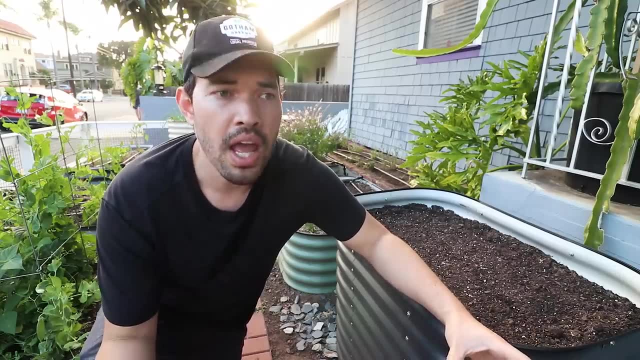 and I was stuck with it and I didn't know any better at the time- and I filled most of the beds that you see here with it. Now they got a decent season of growing out and then it was just completely compacted. The roots couldn't go anywhere. There were nitrogen deficiencies. 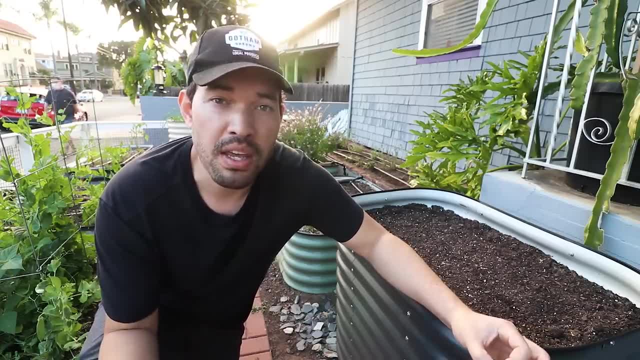 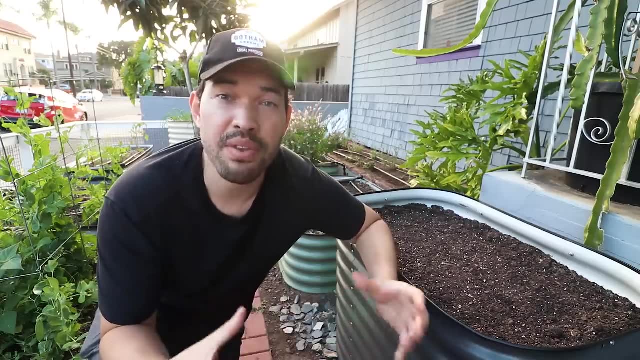 all sorts of problems were happening. So if you're going to invest in something, you should invest in your soil, because we really don't feed our plants, We feed the soil, and then the soil and the life within it is what feeds the plants, And so that's why it's so important, You know. 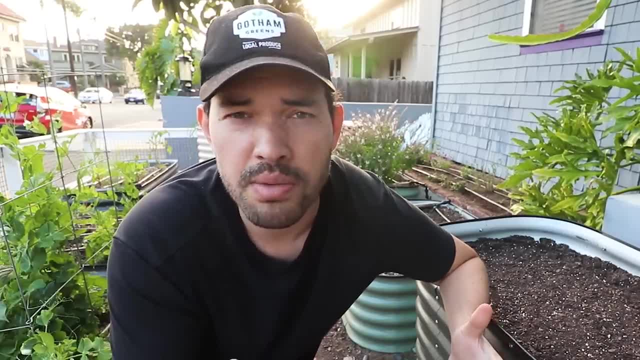 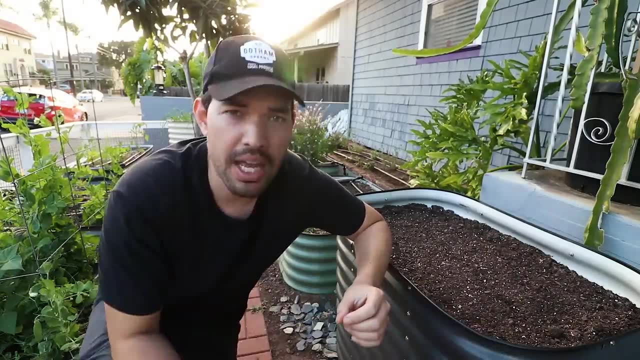 you don't go to a car dealership. really, honestly, who goes to a car dealership these days? But I'm going to continue the metaphor. You don't go to a car dealership. you go to a Maserati and then put a Camry engine in it and say: 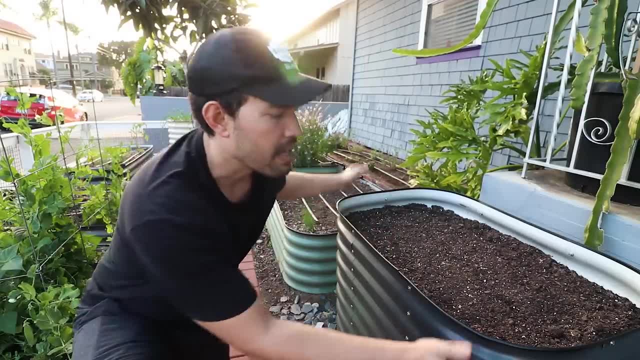 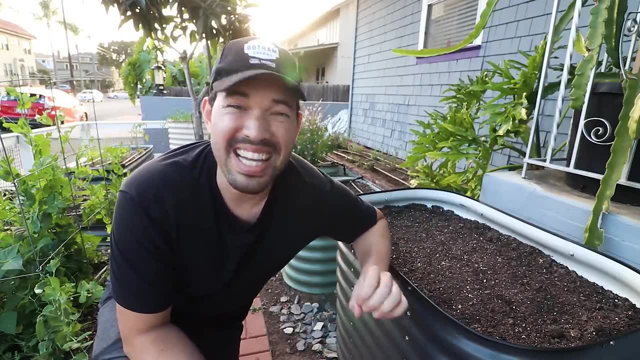 why does it drive like a Camry? That doesn't make any sense. So you don't go buy like a nice high quality raised bed or a nice trellis or whatever and then try to grow plants in that system with crappy soil. It doesn't make any sense at all. So if we don't want to invest in crappy soil, 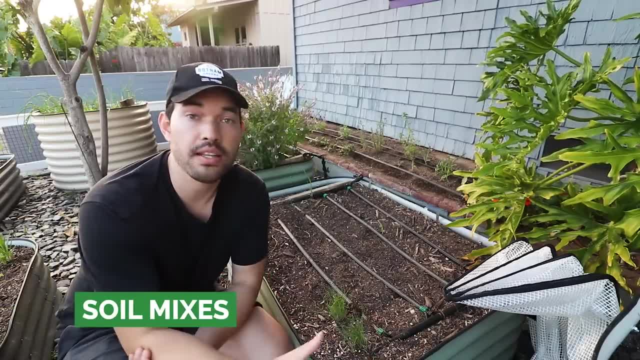 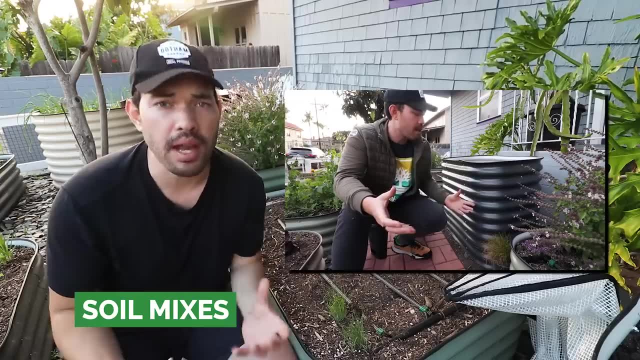 then how do we actually create good soil? I talked recently in a video about how to fill a tall raised bed with soil in a cheap manner, and you can use a lot of the tips in that video, So I recommend looking that up. There's a couple of classic soil mixes that I'll leave in the video description. 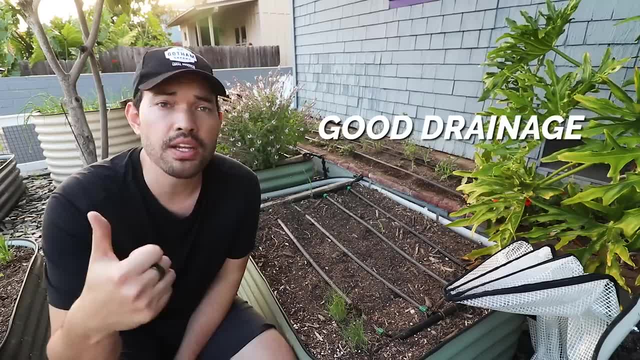 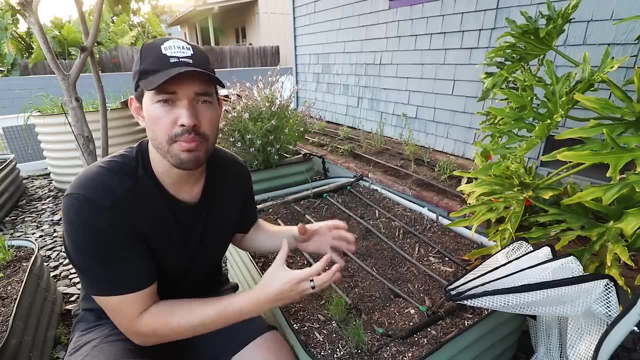 but to suffice to say you want to create something with good drainage, good nutrition and good water retention. So compost, compost, compost- blended sources of compost- should make up roughly one third of your mix. Some kind of aeration component can make up one third of your mix. 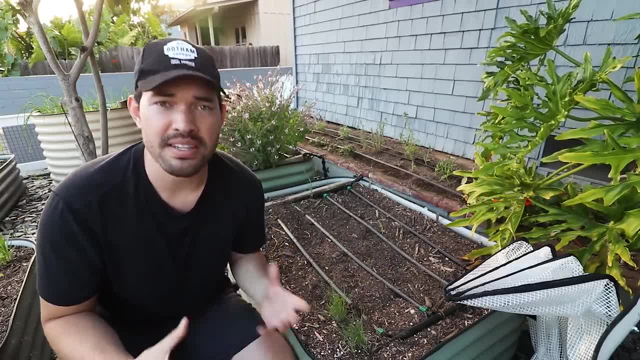 That might be perlite, that might be pumice, some sort of water retentive material like peat moss or coconut coir- Coconut coir- for those of you who are trying to use less peat moss- can be the other third. 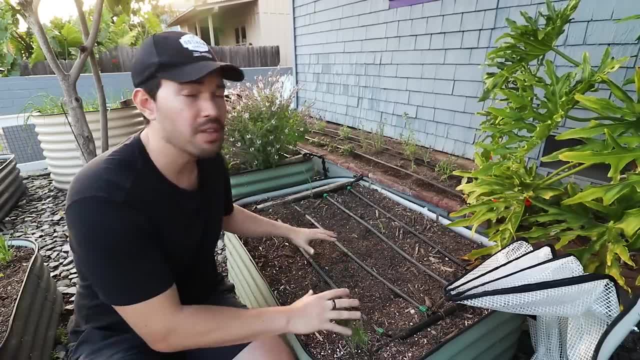 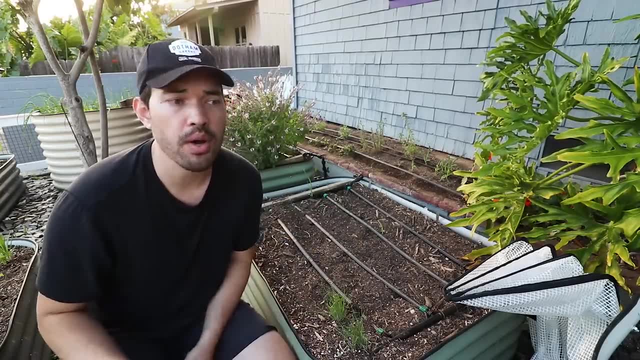 That's a very good all around recipe. If you want to use a lot of your native soil, you may fill around half of a raised bed with native topsoil and then mix in about 25% compost, 25% grass clippings, unfinished compost. 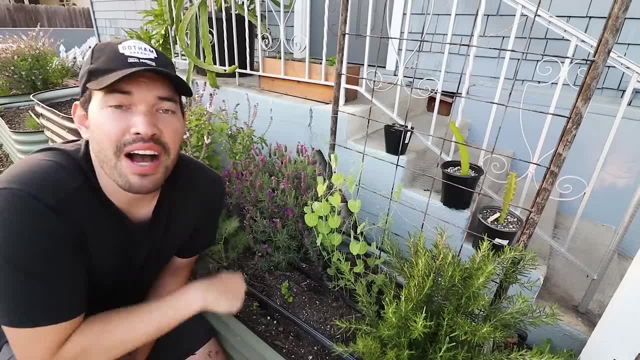 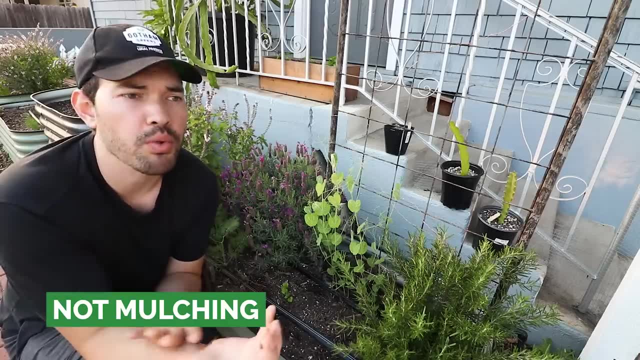 you know that sort of thing. to round it out, Mistake number five, pretty common one, Honestly. it's not mulching. I don't know why. I think it's maybe because when we, as a beginner gardener, we hear the word mulch. 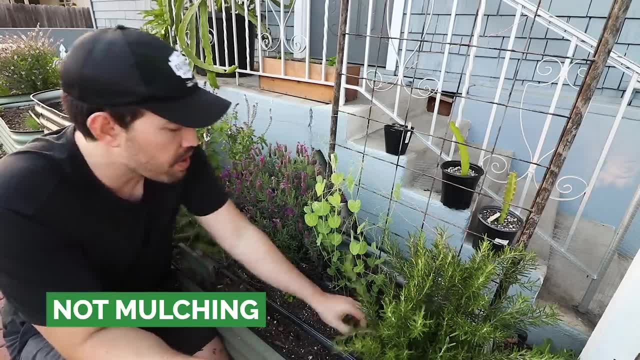 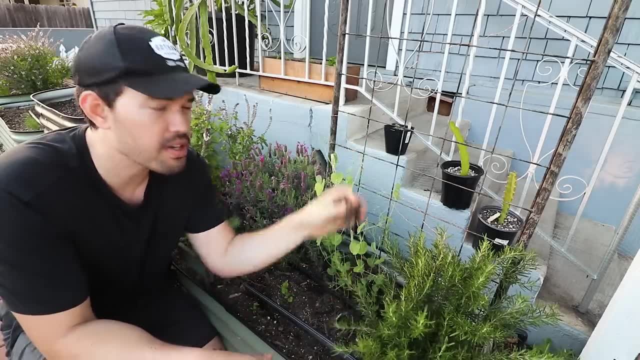 we just literally do not know what that means at all and it sounds weird and so we don't understand it. We don't know what it does. Mulch is basically an organic covering for the top of your soil that's going to protect your soil. It's going to help keep it nice and moist. 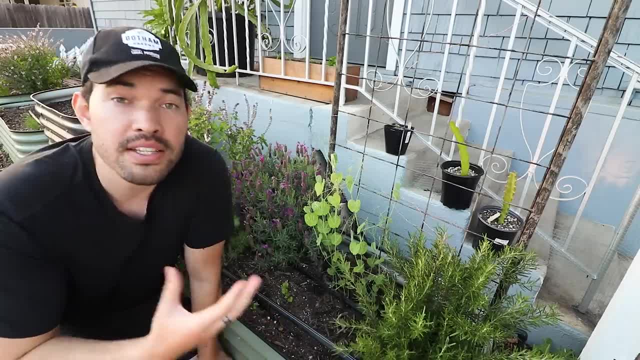 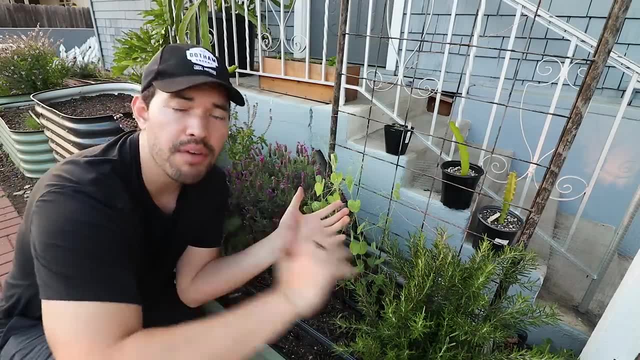 The soil, life will be nice and protected from the sun's harmful rays, It's going to keep water in the soil and overall it just manages the garden a lot better. You can almost think of mulch as sort of a buffer layer to the top of your 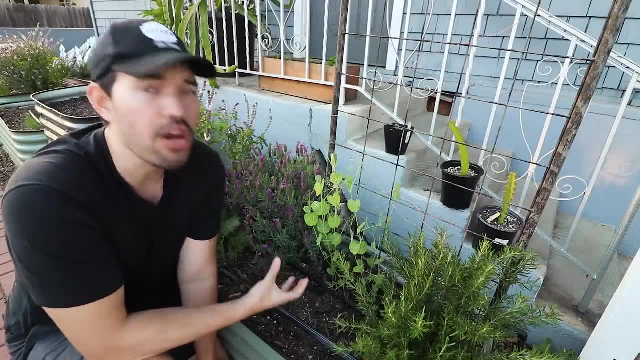 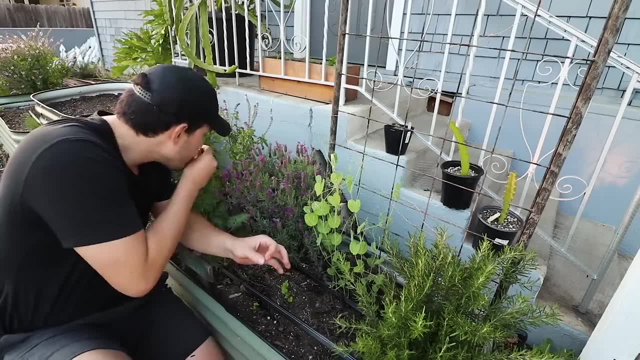 garden soil that's going to really help protect and care for the plants within. So that's why, when I'm filling a raised bed, this is my herb bed and, gosh, it really smells amazing. right now I have this African blue basil. 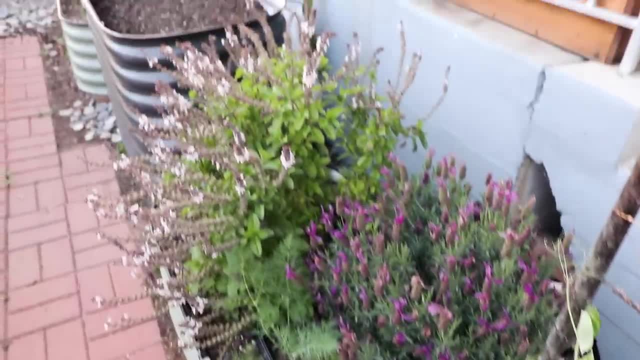 but also the French or the Spanish lavender that's just going off right now. It smells amazing. I wish I could like teleport the smell into the camera for you guys, But what I'll do is I'll fill a raised bed up and I'll leave a couple inches at. 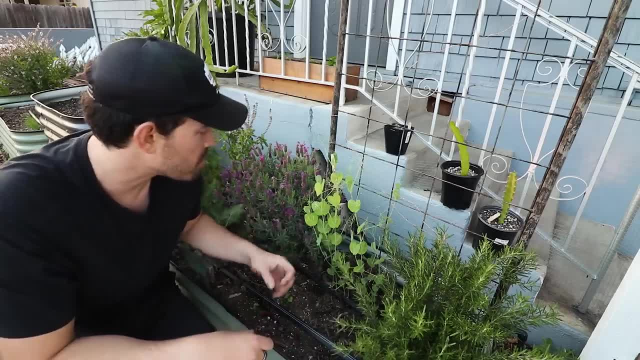 the top and that couple inches will eventually be dedicated to mulch, And so in this bed I've had a skunk kind of come through and dig it up, So I've got to fill it up a little bit more, but I still have to apply, maybe about. 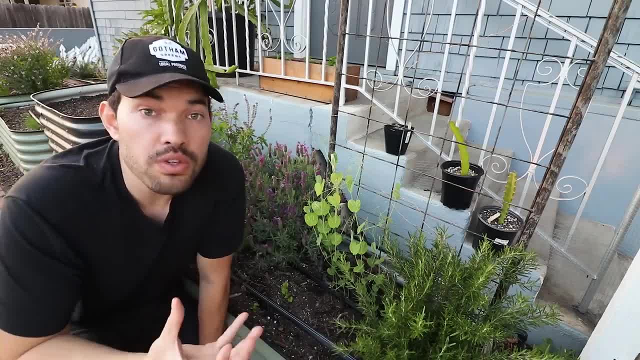 oh, I would say another inch or so of mulch. Now, what sources can you use for mulch? That's really sort of up to you. You can use things like shredders, shredded straw, that's a very good, good source. 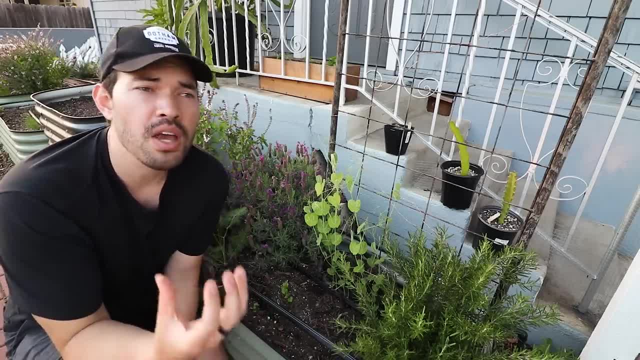 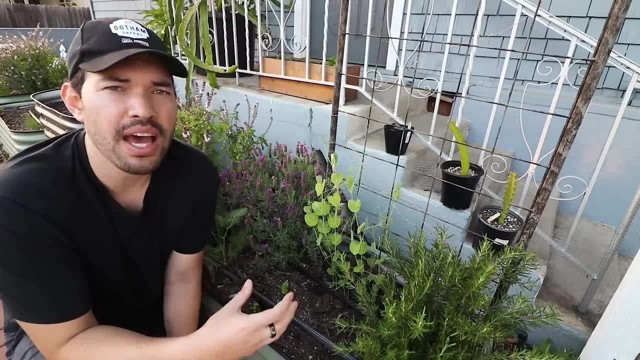 You can use wood chip style mulch, but you just have to be careful, because uncomposted, unbroken down wood chips can actually steal nitrogen from the soil for a little bit until they break down. So if you're going to do that, 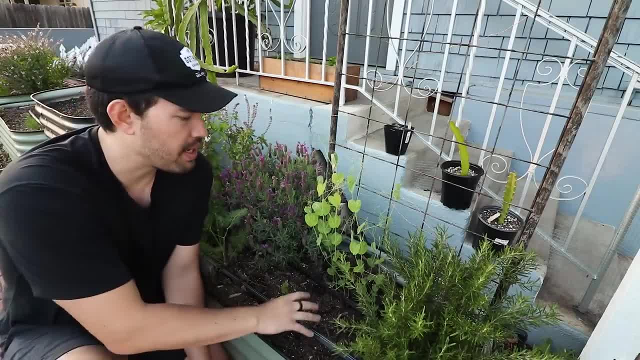 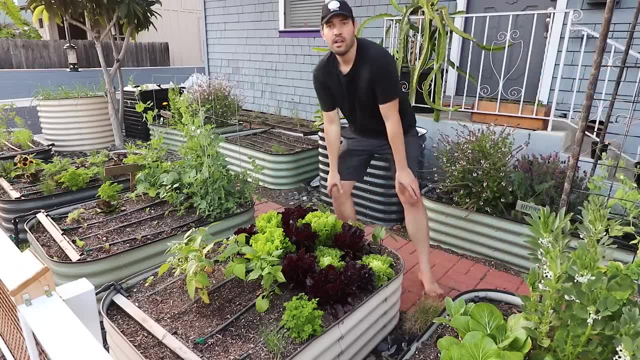 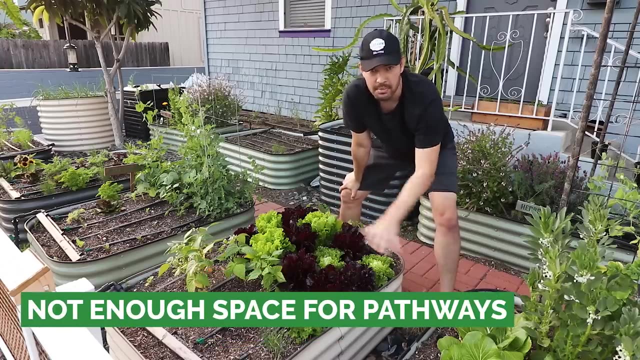 I would recommend not doing it in a vegetable bed or an herb bed like this. Maybe use something like straw or like some sort of more broken down material. Mistake number six is not having a workable spacing between your beds, And this is a mistake I'm currently making on purpose and really follow my lead. 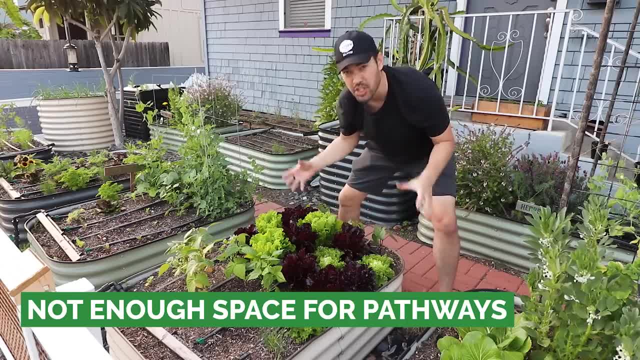 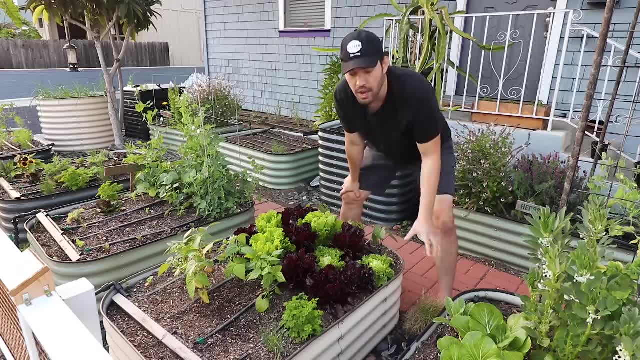 if you want to, but I don't recommend it because I'm really trying to cram as much as I can into my garden so I can show you guys everything that I possibly can in this space. So if you have more space and you don't want to be cramped, 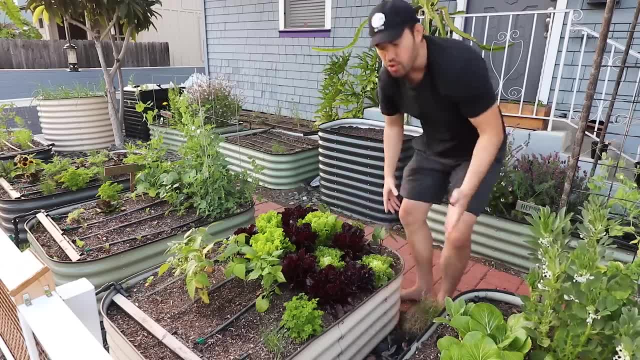 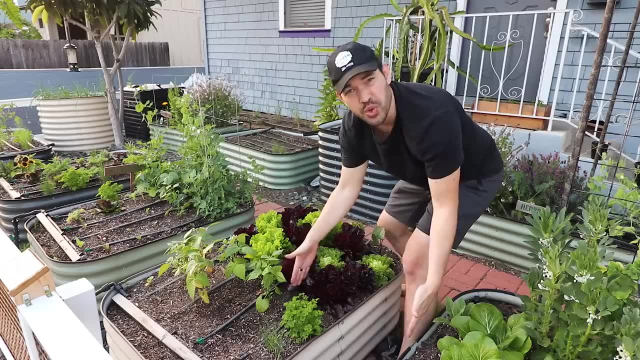 I'm a pretty big guy and I've cramped myself, but usually what you would do is you would leave about two feet. So this is about one foot right there And you would leave roughly two so you can actually walk in and work in this bed. 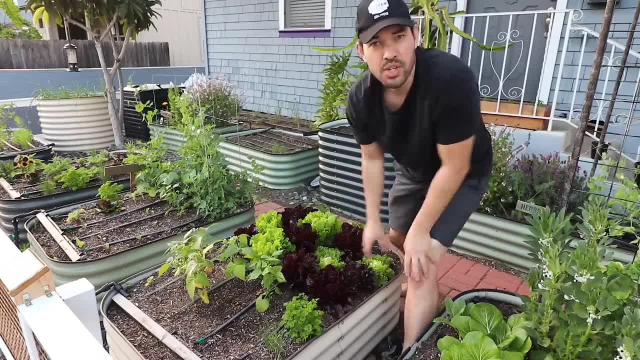 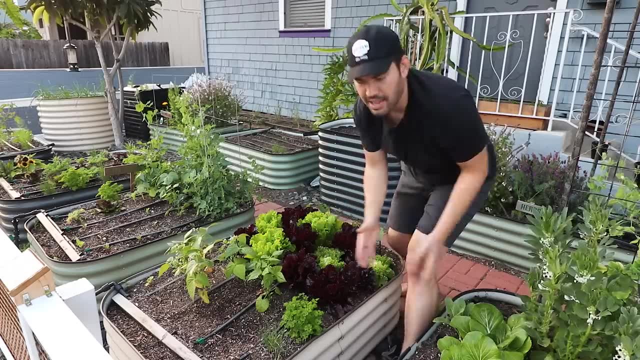 So I kind of have to kitty corner in and make my little ninja moves to do it. but I'm okay with that personally And I knew that going in. but I know a lot of people who've set gardens up. they just didn't think about the fact that they would have to kind of come. 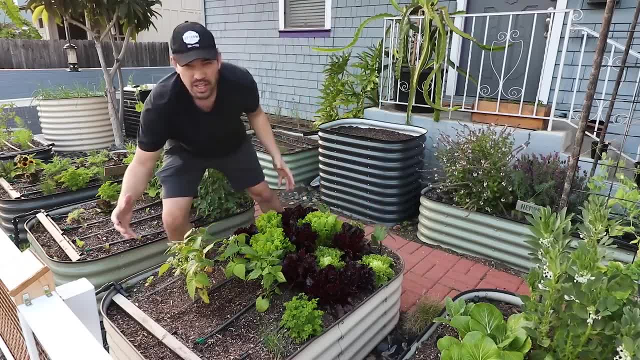 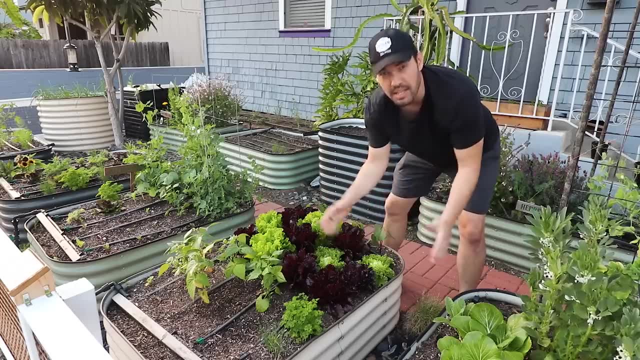 through and work in these gardens and then they get really annoyed And eventually that means that they don't actually work in it. So as a rule of thumb I would say 24 inches or two feet between each bed is a good rule of thumb. 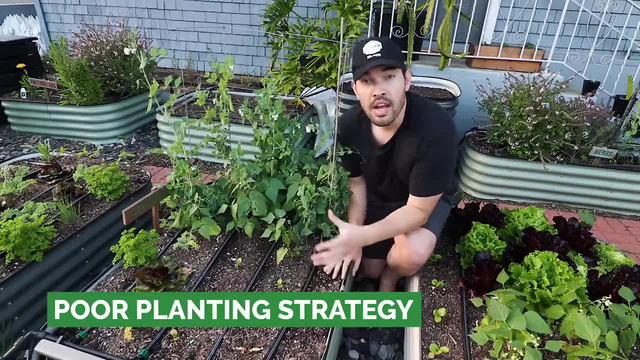 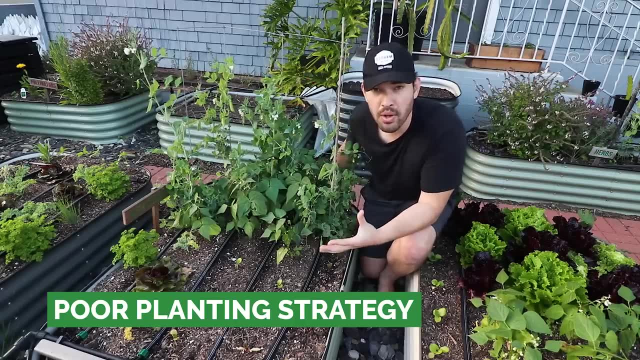 Mistake number seven is when you're planting in a raised bed, not thinking about the eventuality of that plant, how that plant's going to look once it's fully grown. So here's a good example of a way that you can plant a raised bed. Remember: 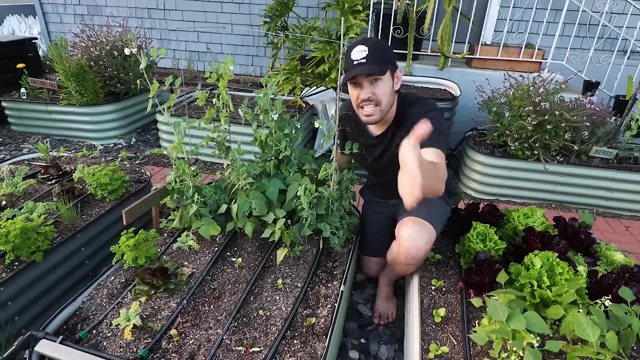 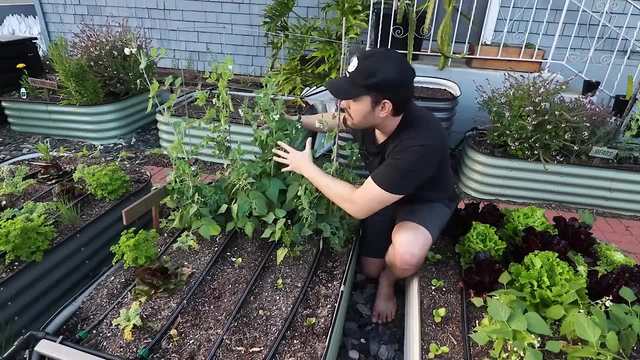 tip number one was placement. South facing is this way, right here, which means that sun exposure is going to be coming throughout the day here, which means that if I was to have planted my peas and beans up front and these newly transplanted in leafy greens behind, 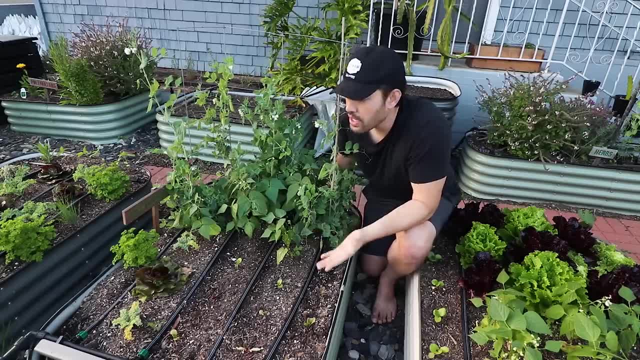 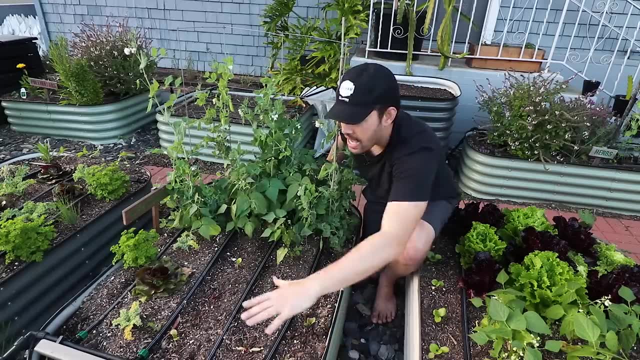 I would have completely shaded them out. I really wouldn't grow that well. So what did I do? I kind of created a little lift here, So I have my low growers up front, AKA on the south side, and then my beans, which are my mid-tier growers. 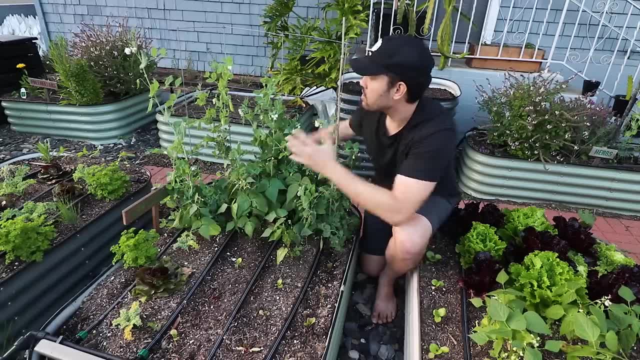 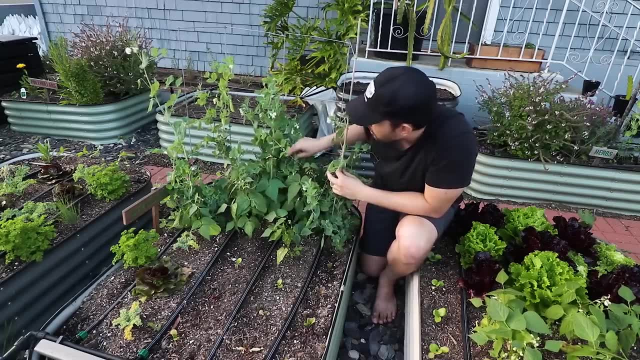 These are bush beans. Those are sort of in the middle And then on the back. you can see, I created kind of a U-shaped, a little funky trellis for my peas, which I've been doing really well. actually, We have all sorts of snap peas going on here. 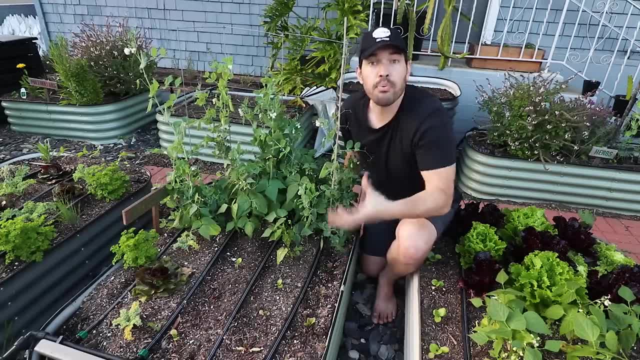 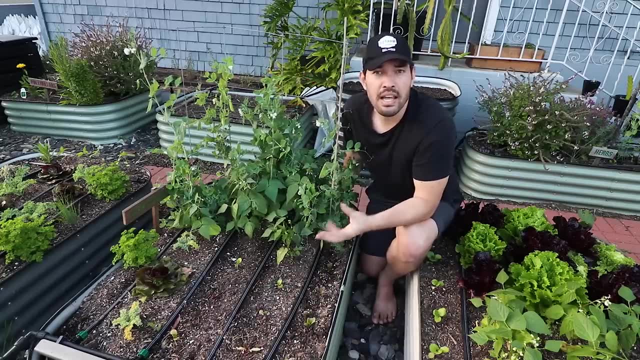 but I've created a bit of a terrace, And so let's say, let's teleport into summer. right, I'm in summer now. Maybe I'm doing onions here, I'm doing peppers here and I'm doing tomatoes here. That's how I would design this bed, And so if you don't think about that, 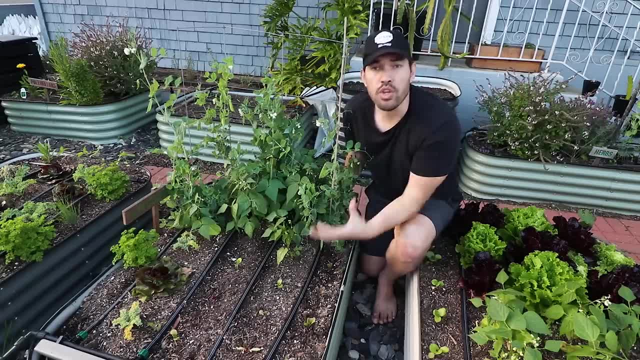 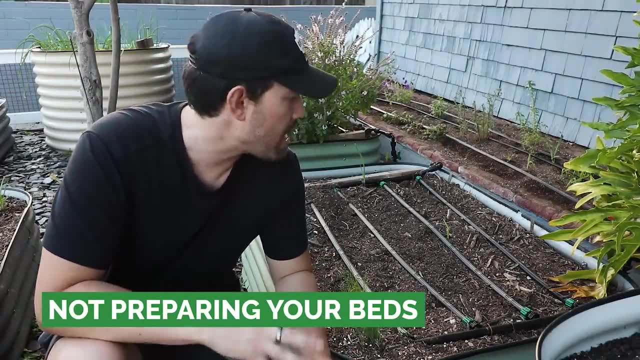 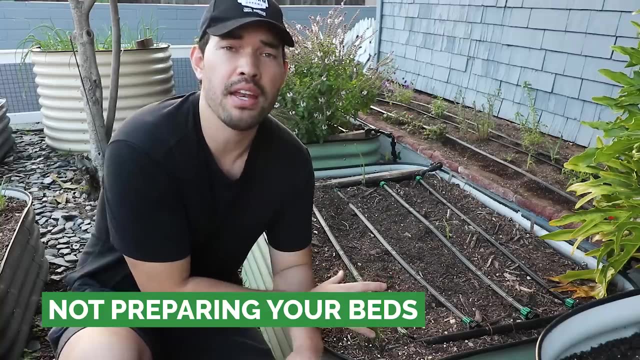 you're just going to be unnecessarily shading and making poor use of the space in your garden. Mistake number eight is bed preparation throughout the seasons, And so as you move into your winter, your fall and winter, there's a couple of different ways you can approach taking care of your bed. 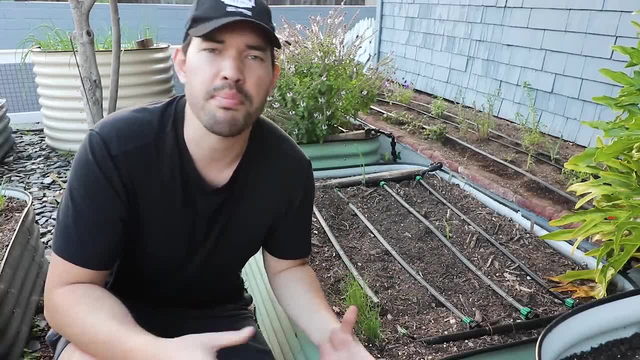 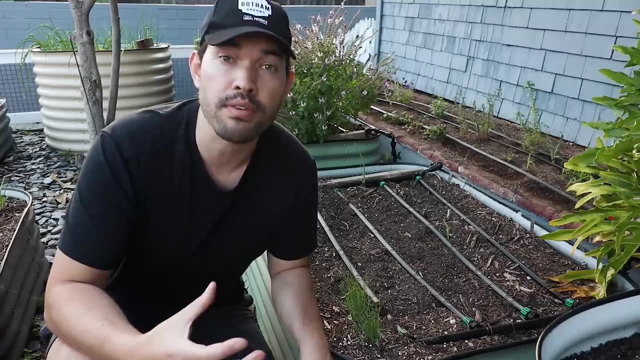 And if you don't do it, you're not going to necessarily fail, but it's just going to be less successful. So with our raised beds, any garden in general, you want your soil to improve, improve, improve, improve over time. 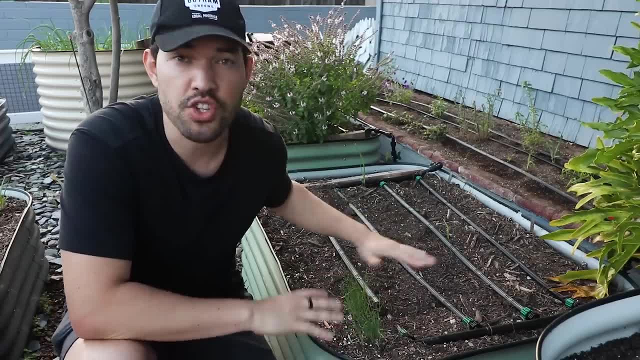 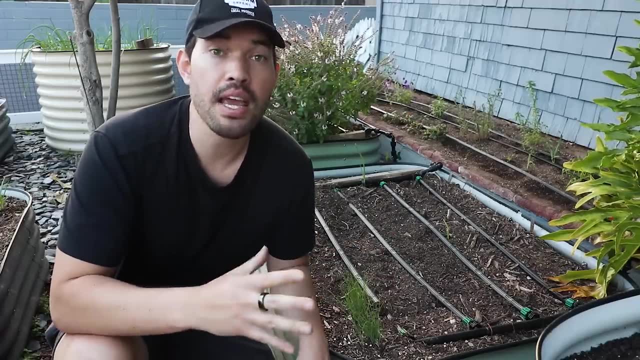 And a bad way to do that would be, as I have in this bed, to just let it be bare when I'm not growing. I just cleared this out, so I'm very quickly going to replant this and amend, But let's say we're moving from fall into winter. A couple of things you can do. 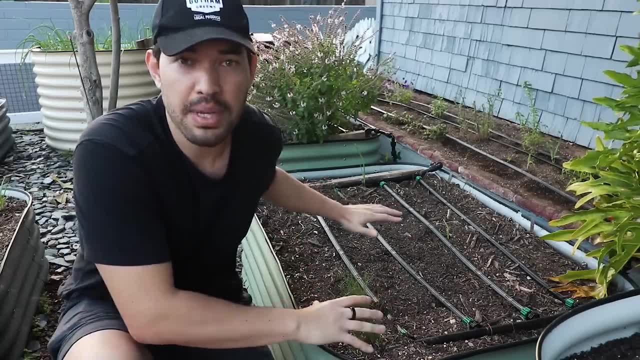 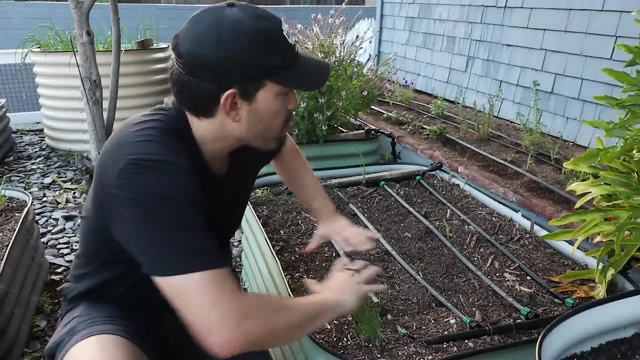 You can just throw on some mulch, a couple inches of mulch, and let it be. You can do what Charles Dowding does and throw a couple inches of compost on and let it be. You can take a cover crop, spread that over. 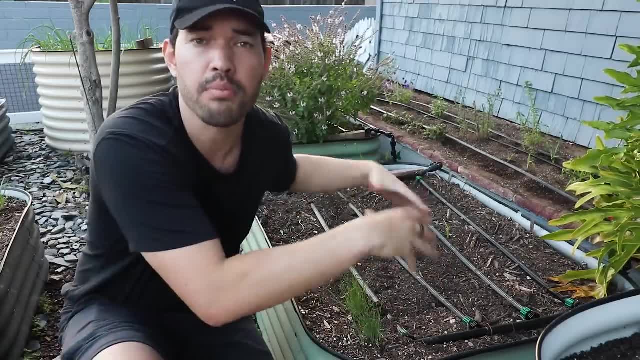 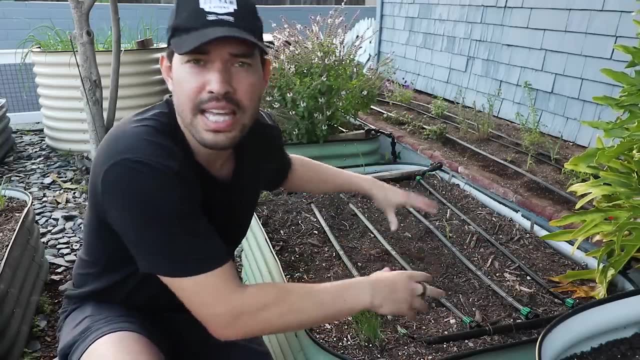 and a cover crop is exactly what it sounds like. It's a crop that covers the soil and protects the soil and then just let that die. in the winter. All of that green material will die on the surface and it will sort of make its way down. There are a lot of different things to do. 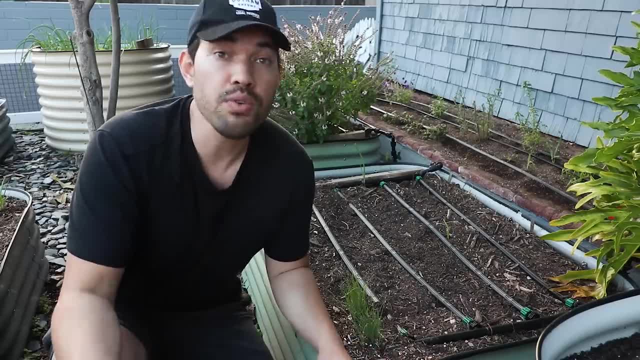 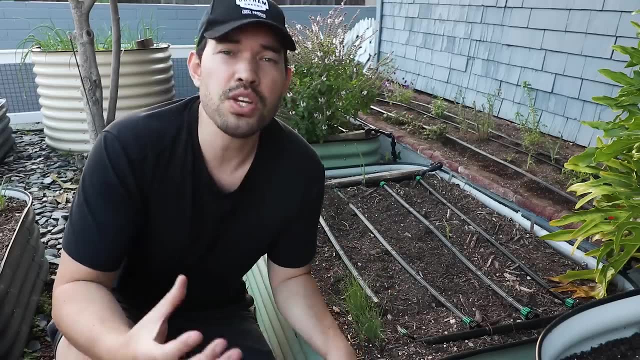 but the thing you don't want to do is just let it be bare And as you move into the spring again. what you can then do is perhaps amend a little bit more before you plant in. You just want to make sure that you're preparing and caring for your bed over. 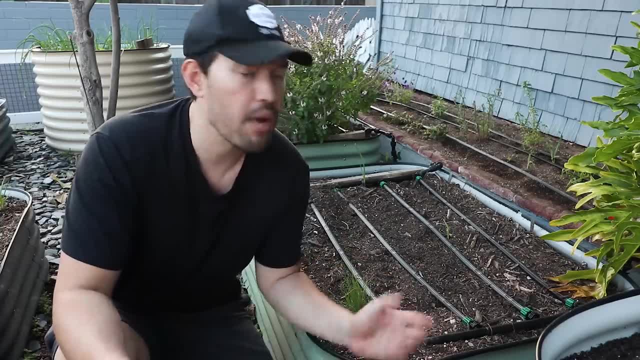 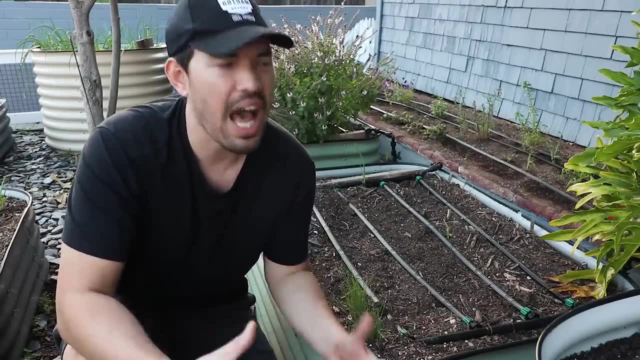 time, instead of just like ripping some stuff out and just saying, okay, well, I'm not going to grow in that for a couple months, I'll just let it be. The sun's just going to beat down on it. The soil is going to become dry and sort of crusty and just not a breeding. 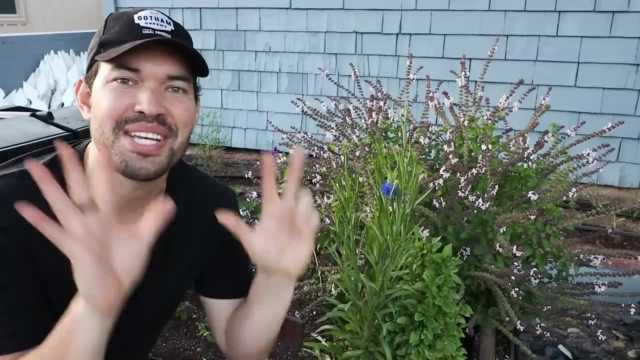 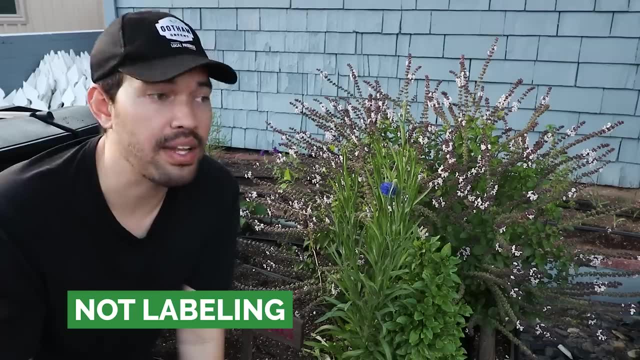 ground for really healthy plants the next time you plant in the bed. Tip number nine, I believe, is not labeling or tracking what you're putting in your raised bed garden Now, unless you're Russell Crowe and you have a beautiful mind or an eidetic. 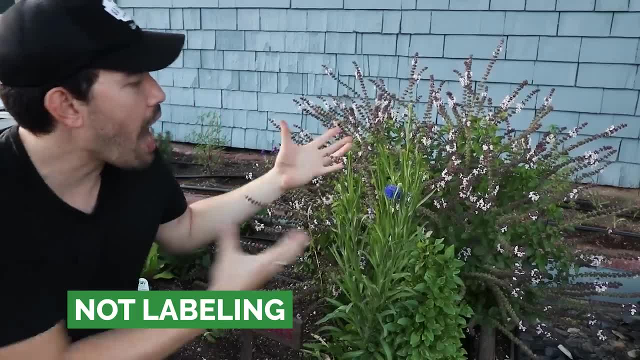 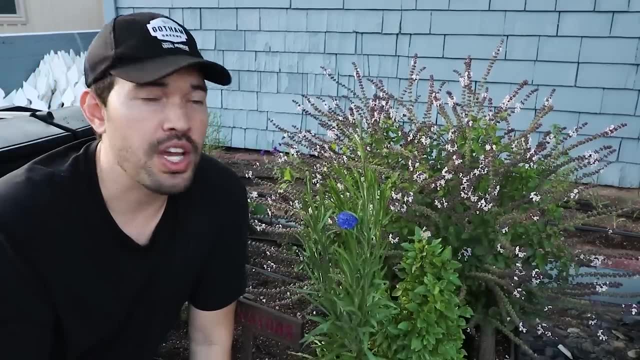 memory of some kind, you have to label and track. you know, Yes, I know, this is African blue basil. I know what I planted: Here's Greek columnar basil, right here. But some of the stuff you just will forget and you'll forget the specific. 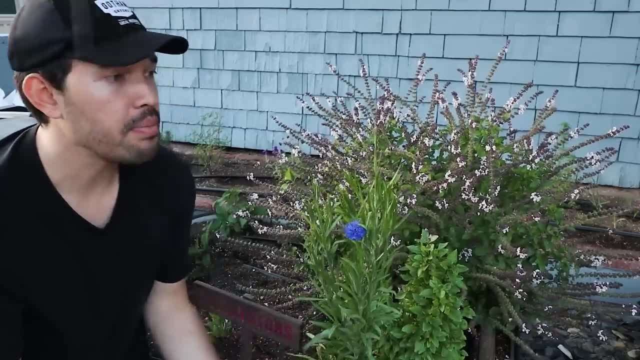 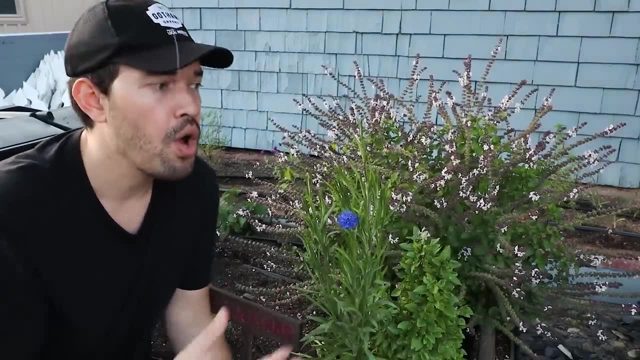 variety and you may even forget when you planted it. And for a lot of plants, when you planted it is much more important than what exact cultivar you planted, because, let's say, for tomatoes or for our peas and beans, you want to know when it's getting ready for that next phase. If I have to start pruning it, if I have to start pulling it, whatever the case may be. So I highly recommend labeling. I'll sometimes, like I do right here with this Amazel basil from Proven Winners. I will leave these in. 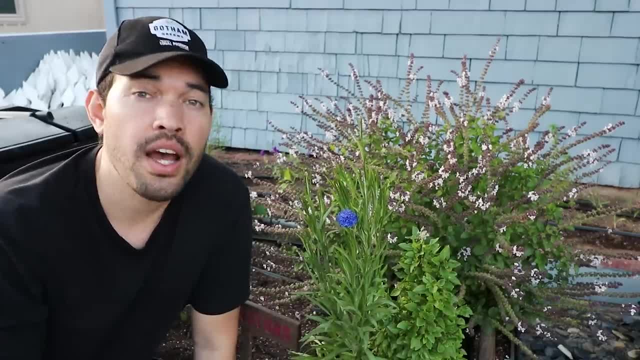 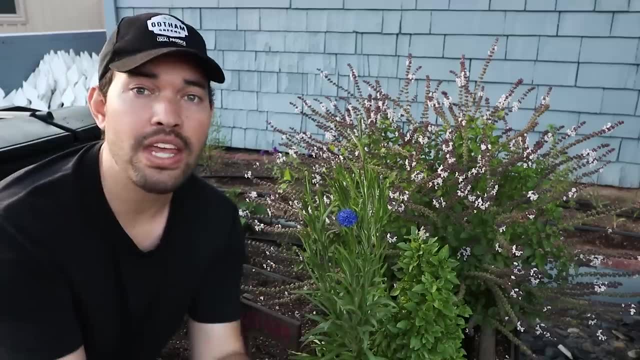 But a lot of the times I just have a little Google sheet on my computer. You can draw it out on graph paper, It doesn't matter, It's just the method. I'm agnostic to the method. The way you do it is the way you do it, as long as you do it and you're going to.